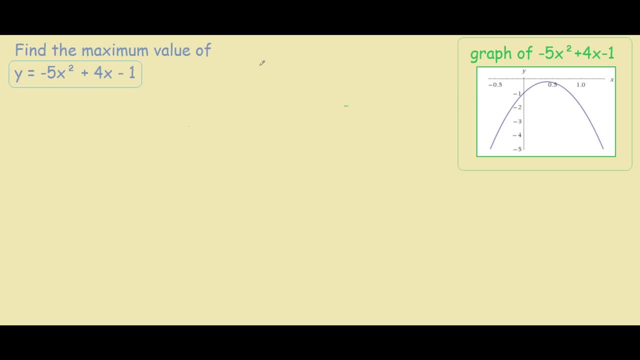 To find the maximum value of a function. you can solve it in two ways. You can do the first way of looking at a graph and then trying to find a peak, or you can do it another way, which is algebraically, by finding dy, dx and equating dy dx to 0.. 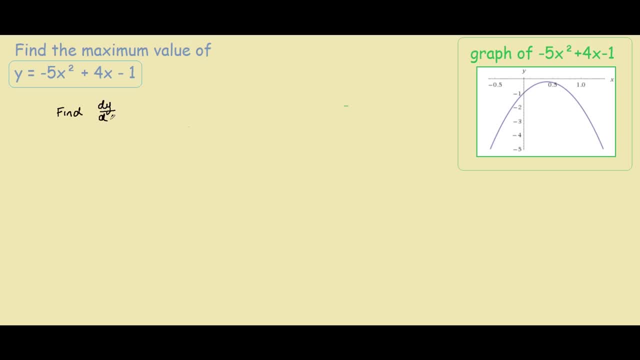 This is because dy dx gives you the gradient function, so the gradient function gives you the gradient at some point along the graph, And what 0 gradient means is that it's completely flat, and this is where the peak occurs, because at the peak the gradient is 0.. So if we find dy dx of this value, we can solve it by looking at a graph and then trying to find a peak, or you can do it another way, which is algebraically, by finding dy dx and equating dy dx to 0.. 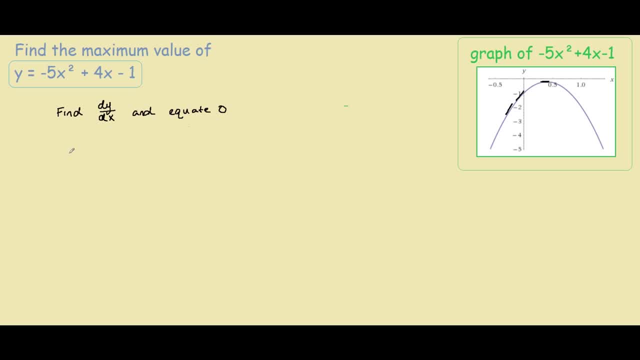 So if we find dy dx of this equation, we get dy dx equals to negative 10x plus the derivative of 4x is 4.. So now you want to equate this dy dx to 0, so we have negative 10x plus 4 equals to 0. 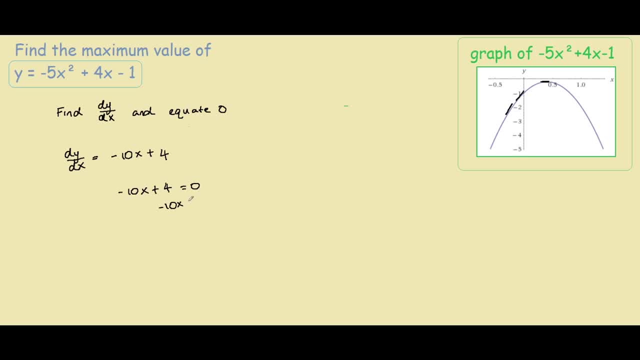 So if you rearrange this, you get negative 10x equals to negative 4,. therefore x equals to 4 on 10, which is the same as two-fifths. So what this tells us is that the maximum value occurs at two-fifths. 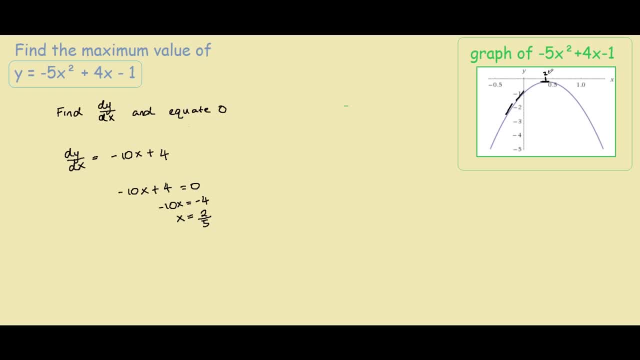 So if we were to graph this, it would be here: two-fifths. And now to find the maximum value, we substitute x equals to two-fifths back into the function. So we have y equals to negative 5 times two-fifths squared plus 4 times two-fifths minus 1.. 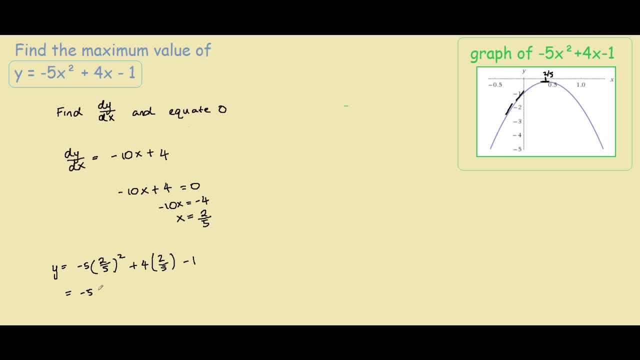 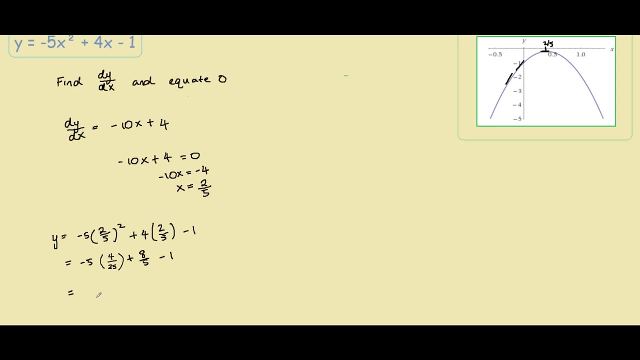 So what is this? Minus 5 plus 4 times 2 is 8 on 5, minus 1.. So actually, if you solve this whole problem here, it would equal to negative 1-fifths.